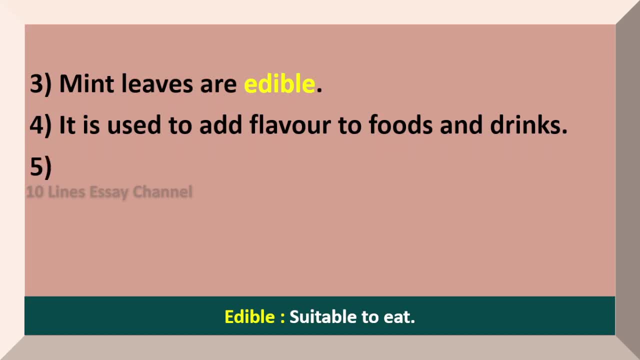 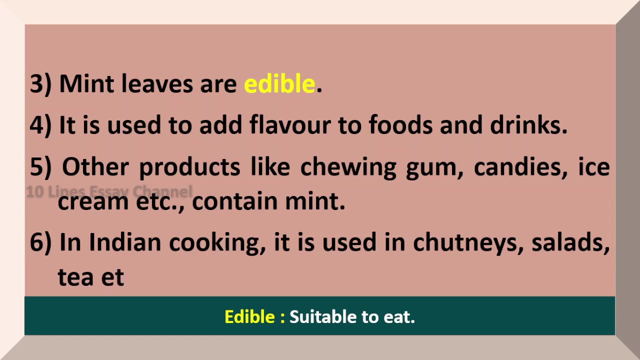 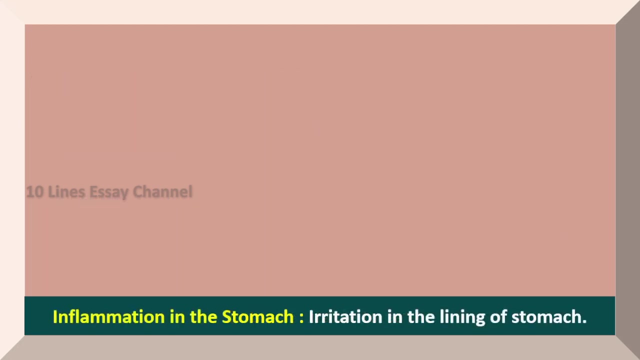 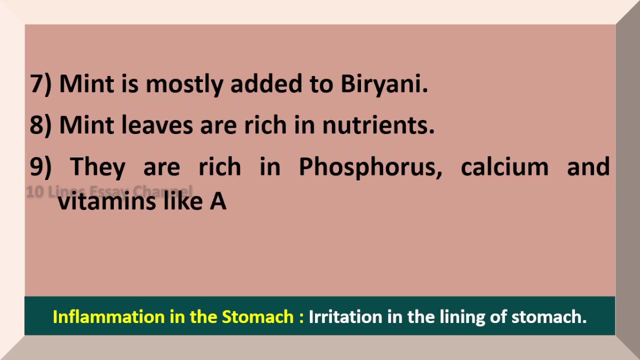 Thanks for watching. Please subscribe to my channel. Thanks for watching. Please subscribe to my channel. Thanks for watching. Please subscribe to my channel. They are rich in phosphorus, calcium and vitamins like A, C, D and E. Minclase is used to mix.